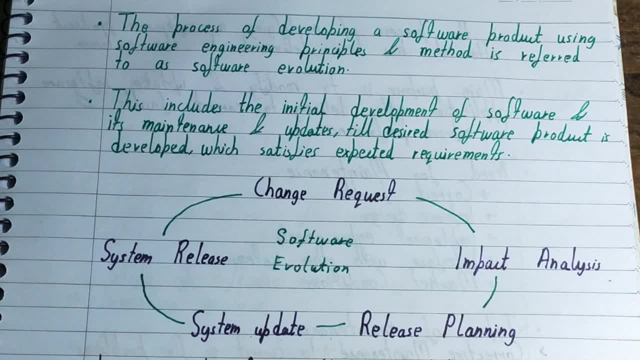 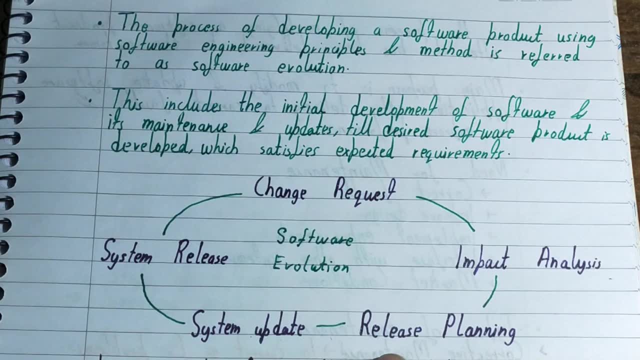 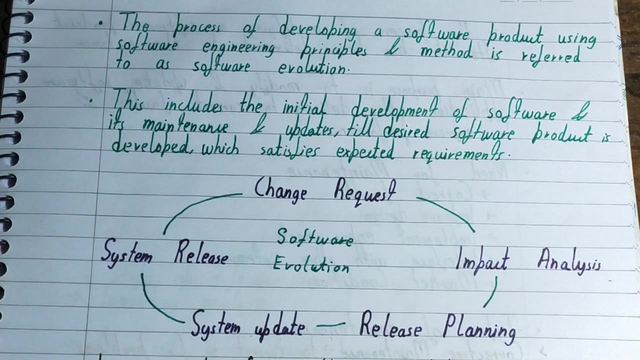 That, what impact it will do If you will be developing those changes, or if you will be doing those changes, then what will be the impact? And according to that impact analysis, you do the release planning of the software And once you're done with that, you upgrade your system or you update your system and you just release the system, Okay, in your real time environment. So this is the lifecycle of software evolution: that how a software is evolved during the development of a software. 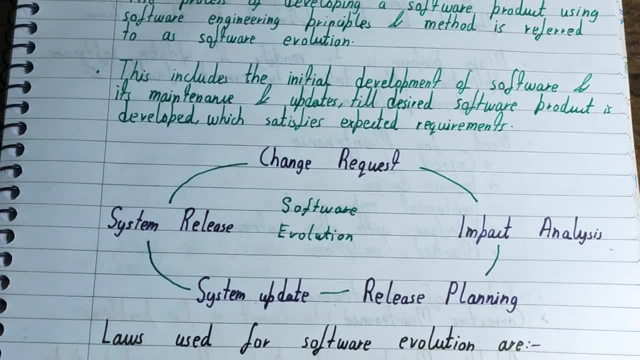 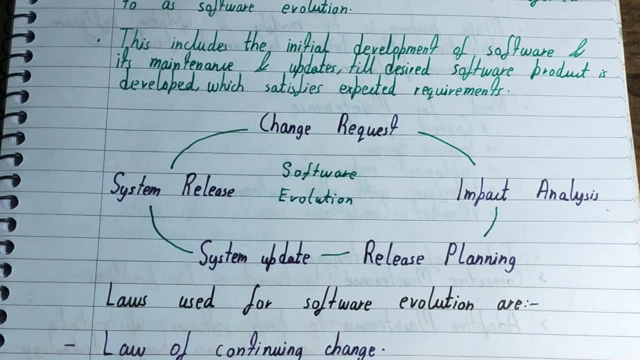 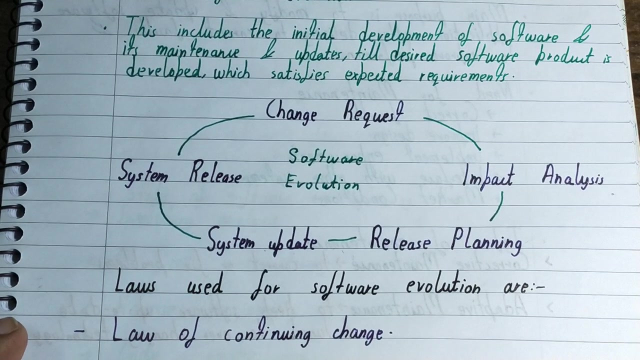 So there are some laws which are followed during the software evolution. And what are those laws? First is law of continuous change. That means if you're developing a software, the software will always be prone to changes over time As the time goes on. the changes will also go on because technology is developed day by day, So that is a daily thing, or you can say regular thing. Next is law of increasing complexity. So as the time moves on, we are 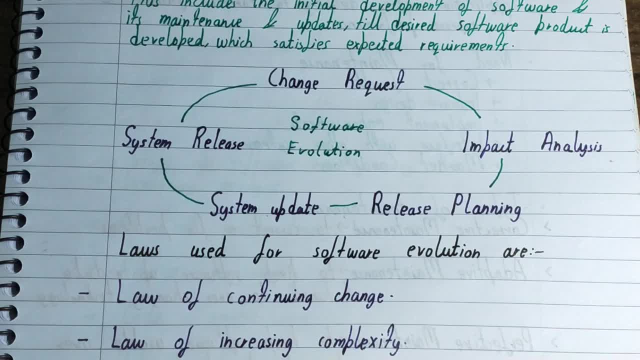 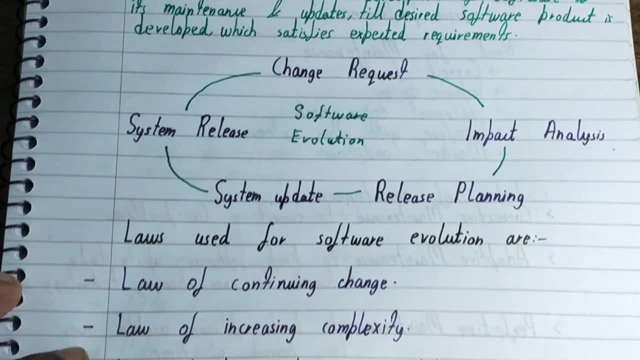 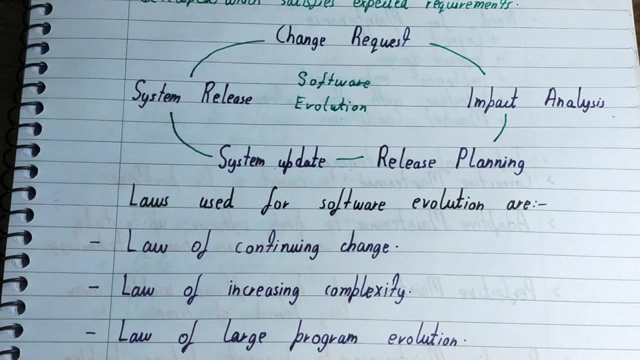 we have seen that the complexity related to software has increased largely right, And over the years it will increase more. So that is also a low. And next thing is law of large program evolution. So when you design a software, it has a limited number of line, right, And it is a very compact software. But as the time moves on, as the time goes on, that particular software goes through various change requests or various modifications. 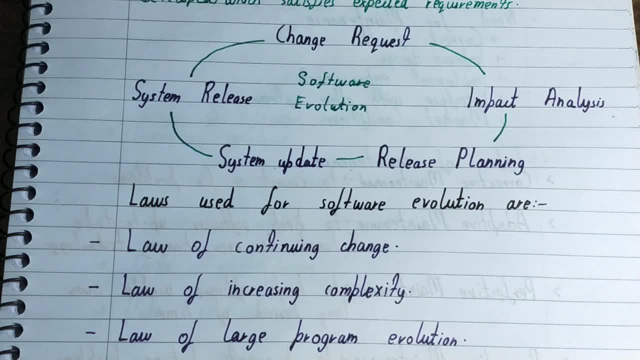 or various changes, right, And upon the changes or modification, that software starts becoming larger and larger and larger. So you can take an example of a very good gaming app like PUBG right. So when it initially released, it was around 1.2 GB or so And presently, due to updates and due to new new modification, that came up to 1.8 or even 2 GB, right, And in near future it will increase more, Same with other gaming apps.